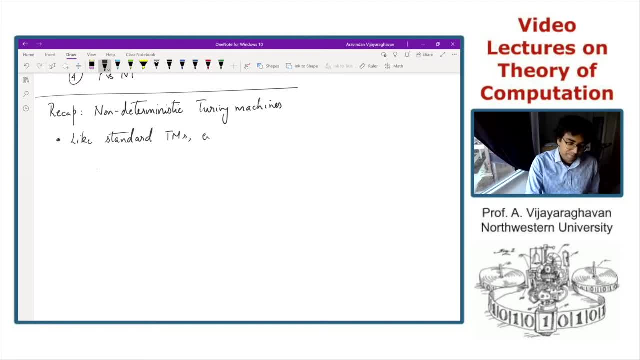 okay, except that the machine can proceed according to several possibilities Here in a particular state of, I mean, and the input symbol and so on, there can be multiple possibilities that the Turing machine can take, And so the machine can proceed along these different possibilities. Okay, and the non-deterministic Turing machine accepts a string. 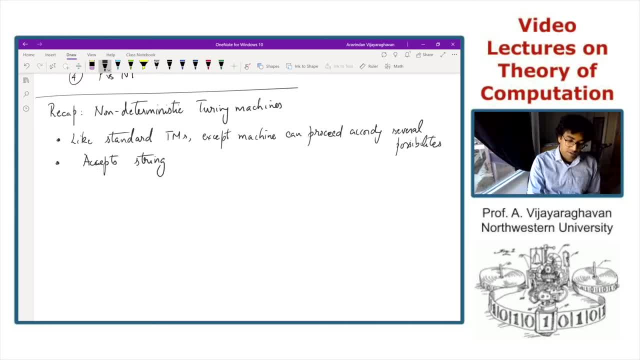 if there exists an accepting path. So this is very much like a nondeterministic, finite automaton, except that this is just the same in the context of Turing machines, where you have a tape as well. So there should exist a path from the starting configuration. 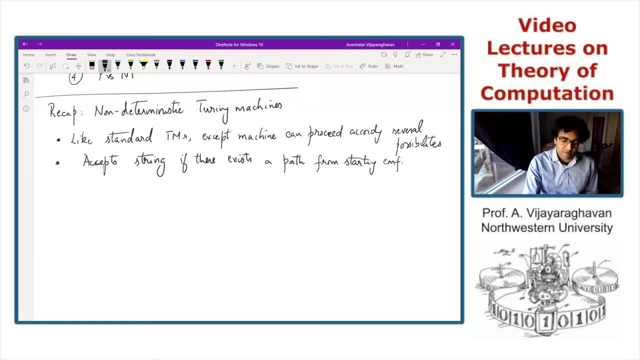 or a sequence of moves from the starting configuration to an accepting configuration. There might be multiple sequence of steps that you can take. As long as you have one sequence of steps that go from the starting configuration to an accepting configuration, that particular input is accepted. 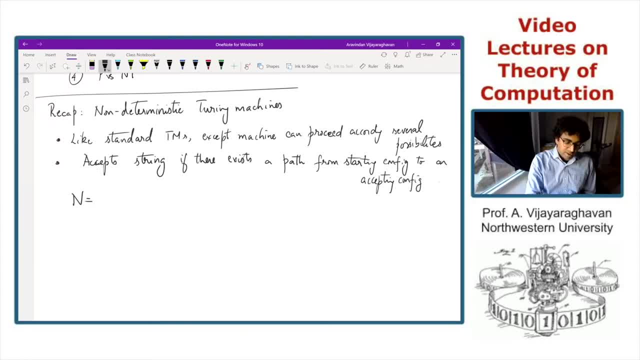 So the nondeterministic Turing machine will also be represented by the usual 7-tuple And you have the usual set of states, the input alphabet, the tape alphabet, and then the transition function start state and the set of accepting state. 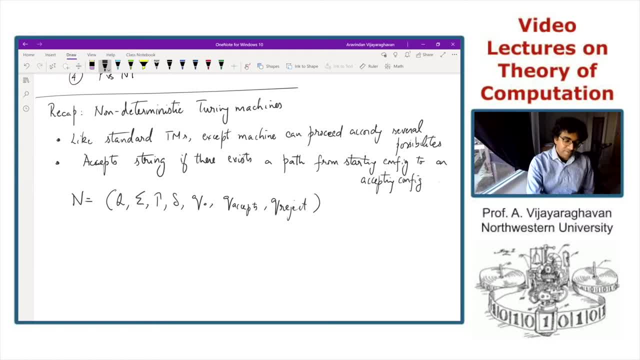 and the reject state. And the main difference is in the, the transition function. This transition function as opposed to a deterministic Turing machine. this transition function- this is just a recap, So it can go from a state comma input pair to a bunch of possibilities. 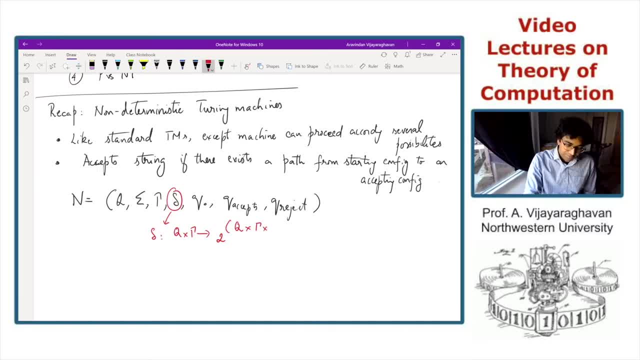 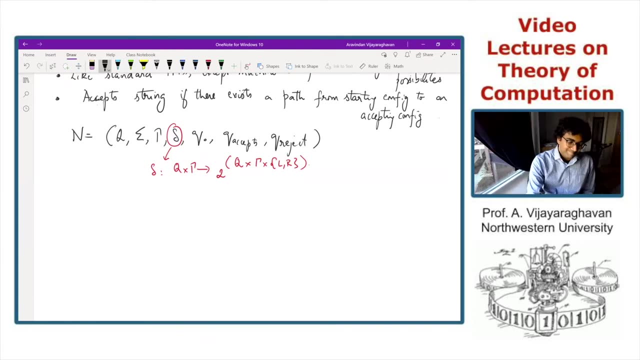 So this is represented as a power set, A set of possible moves, A set of possible moves. So you would find some set of possible moves. so you would find some set of possible moves. Good, And just to kind of pictorially keep this in mind. 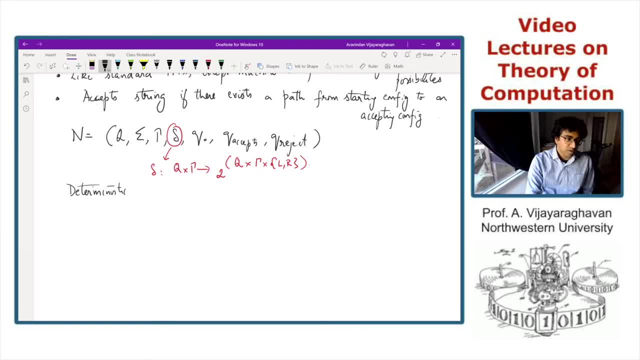 in a deterministic Turing machine you start with some start state And then you take a bunch of transitions given by the input and so on, OK. So initially you start with Q0 and some input, W- OK, And then you take a bunch of sequence of moves. 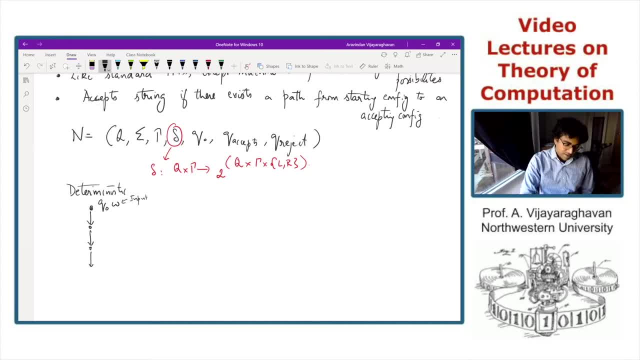 And finally, you end up at some table, or you end up at some table, or you end up at some table, And then you take a bunch of sequence of moves And finally configuration, which is either an accept or a reject. okay, we are. we are mainly looking at. 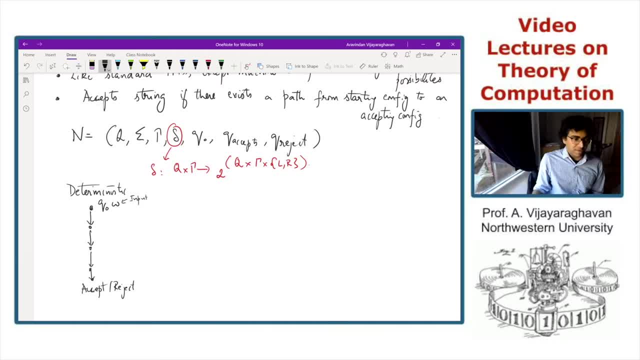 decidable problems- so we can assume that the turing machine always accepts or rejects- versus a non-deterministic computation where you can start out with this configuration of initial state and input and then you know there might be multiple possibilities. so maybe the first step is fine, but then you may have start seeing multiple. 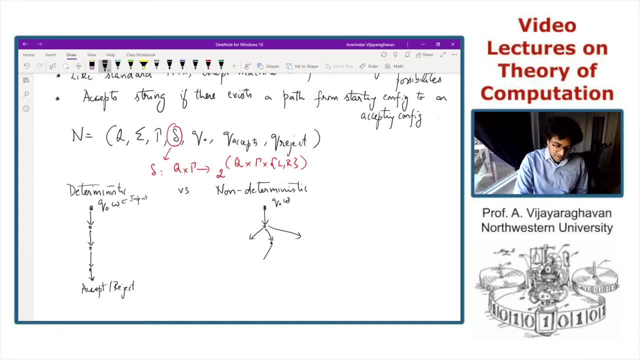 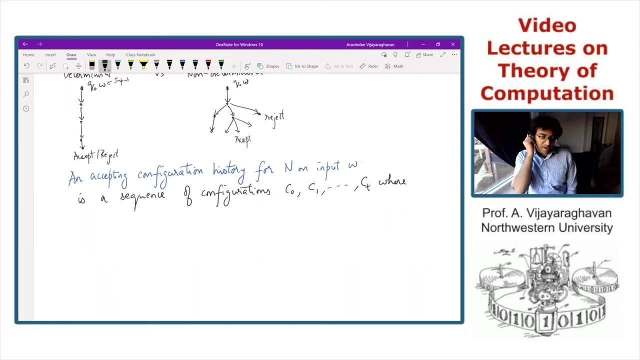 possibilities and, in turn, you may see multiple possibilities here and so on. okay, and some of these could be accept configurations, some of them are reject configurations, some of them are accept configuration. okay, now let's go a little more into detail about accepting configurations. okay, in particular, let's define what is an accepting. 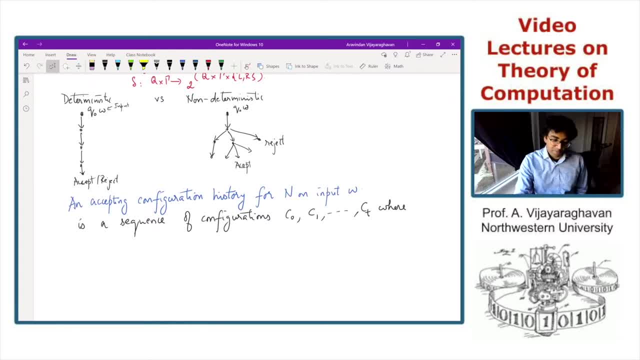 configuration history for the non-deterministic turing machine n that we have defined here. okay, on input w. so an accepting configuration history. it's a sequence of configurations, okay, 2 up to CT, where C0 is the start configuration. So for instance, here it's a starting state. 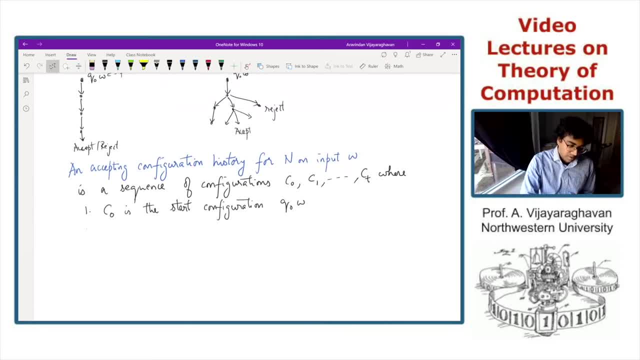 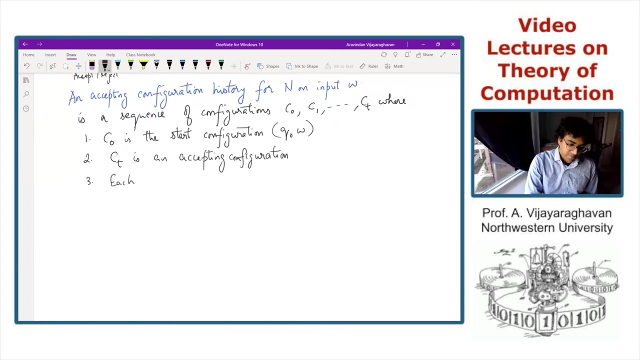 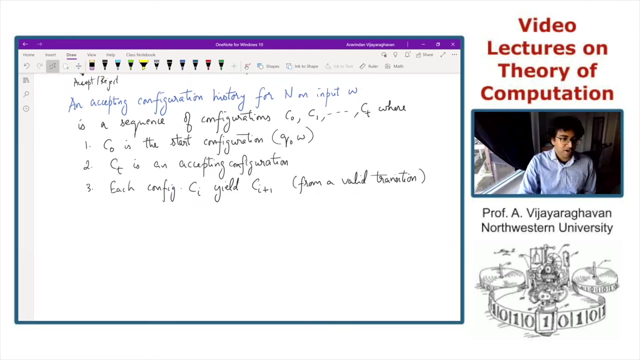 is Q0 and the string is W, CT is an accepting configuration. And finally, each configuration CI yields CI plus 1, again from a valid move, from a valid transition. So, if there is such an accepting configuration history for the non-deterministic Turing machine N on input W, 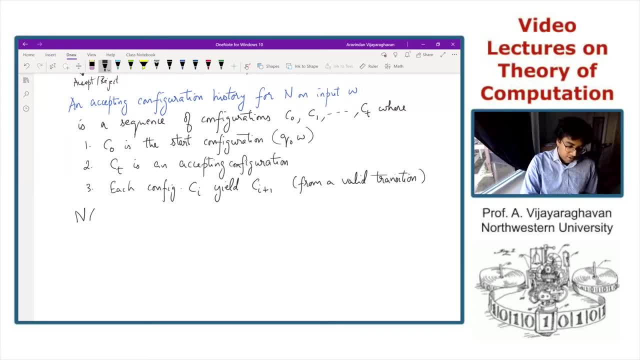 we'll say that N of W accepts. So N accepts W in time T Because it goes from C0 to C1 up to CT, so it's T time steps. So basically enough: W accepts in time T means that such a accepting configuration history exists. 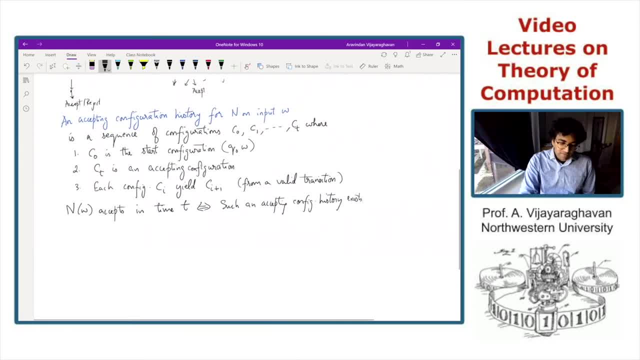 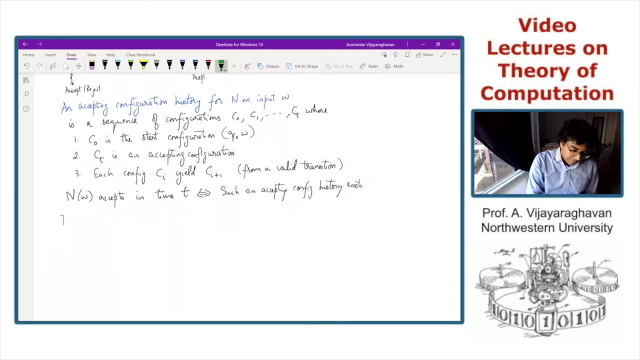 OK, good. So now, just as we defined time complexity of a deterministic Turing machine, we can also now define- you can also now define- the time complexity complexity of a non-deterministic Turing machine in a very similar way. we'll say that N has time complexity, T. 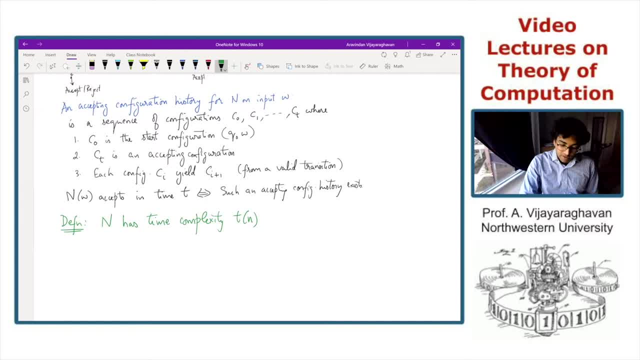 of N, If for all input size, for all N, that is so for all N and for all inputs of length N. so N here is a natural number of length N and all histories, whether accepting or not all histories, and then 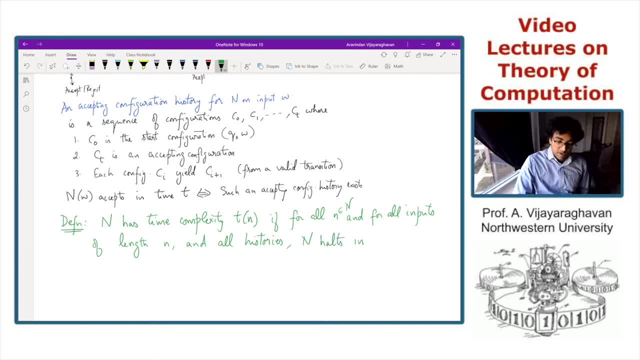 so N halts In T of N time. OK, So the set of configurations that it goes through, that is the history configuration history or computation history, And for any input of size N, the set of all possible computational histories, should really end within T steps. 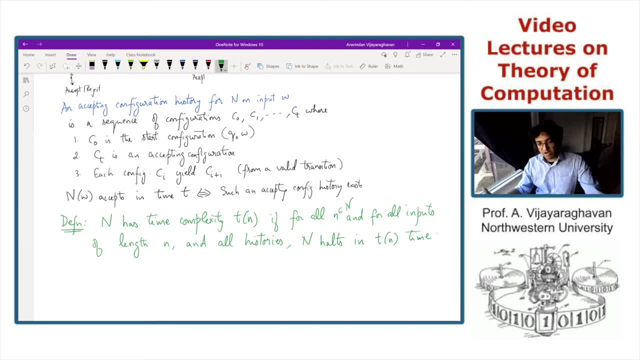 T of N steps. So the non-deterministic Turing machine halts in T of N time. I mean whichever configuration history or computation history you look at, whichever of the many different paths it can go through. Again, this is not really a big restriction. 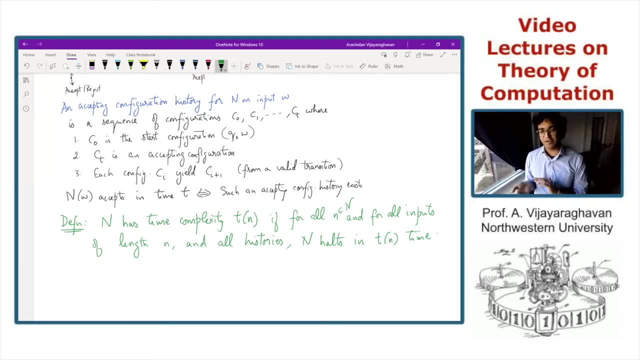 because we are looking at decidable problems. You can always make the non-deterministic Turing machine halt in T of N steps like a clock. Good, So this is the. This is the definition of time complexity for a non-deterministic Turing machine. 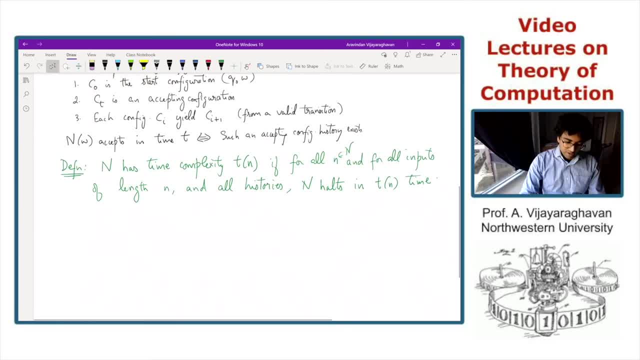 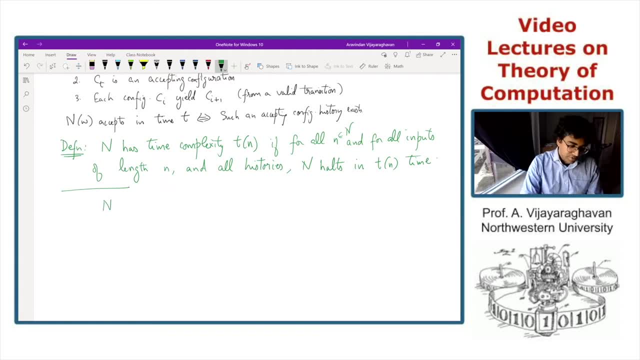 And just like we did with deterministic complexity classes, you can also define non-deterministic complexity classes. So let's say N time. T of N is just the set of all languages. So I said L can be decided by A non-deterministic Turing machine. 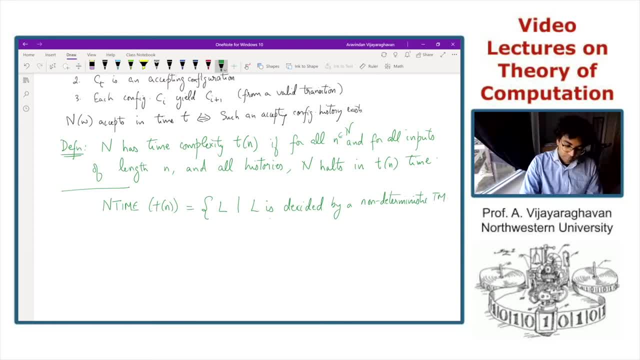 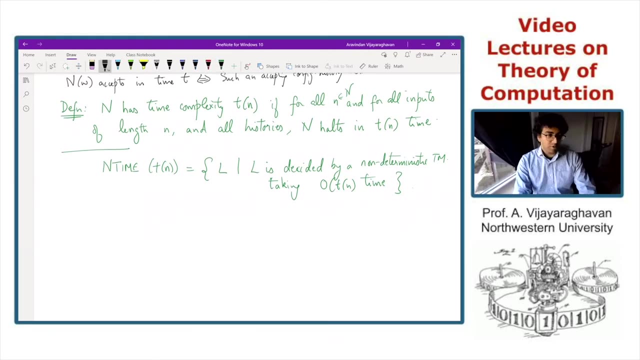 Okay, This takes order T of N time. Okay, Good. So now, if you compare this to ai, which is the number of games, you're going to get a little more time, right, Because this is the kind of time that people use each time. 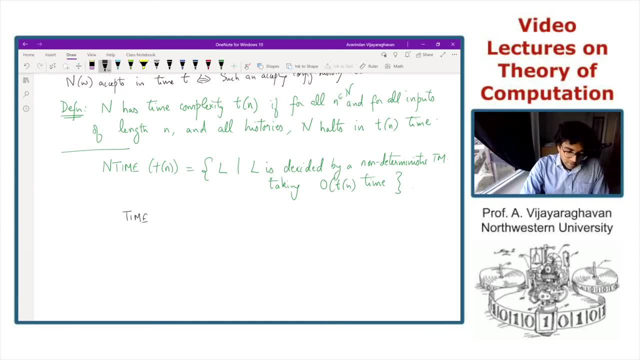 You're going to get a lot of time. You're going to get a lot of stuff right. the two definitions: it's easy to see that the complexity class time of t- I mean t of n- is certainly a subset of the non-deterministic time. complexity class n: time of t of n. 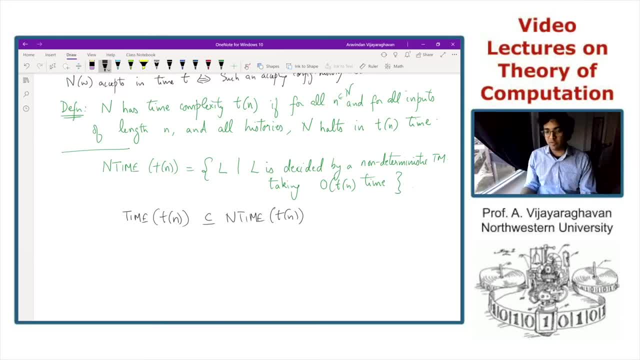 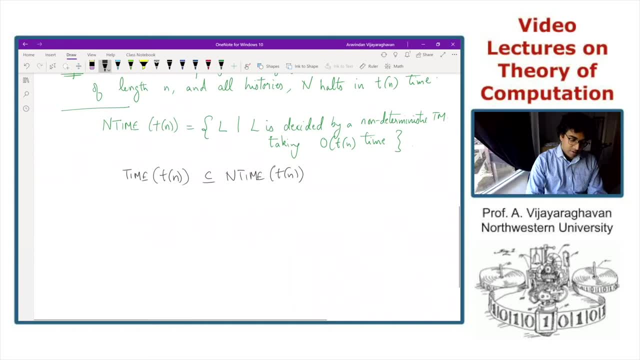 Okay, and why is this? That's just because any deterministic Turing machine is also a non-deterministic Turing machine. Okay, now here is a question that is quite open. Okay, is this a proper containment for all t of n? Okay, and this is still quite open, except for some corner cases. 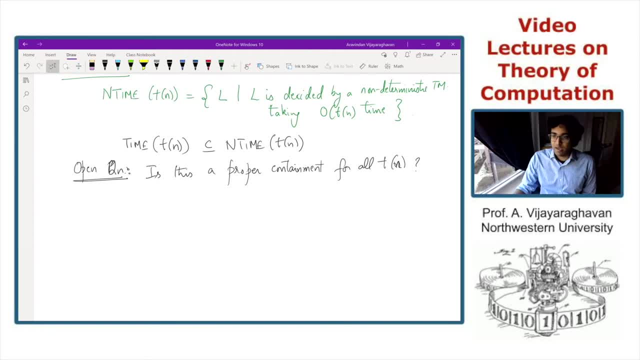 Okay, good. So the next question you may ask is: well, what kind of problems can be solved efficiently using a non-deterministic Turing machine, or what kind of problems can be solved efficiently non-deterministically? Okay, and now let's see an example. 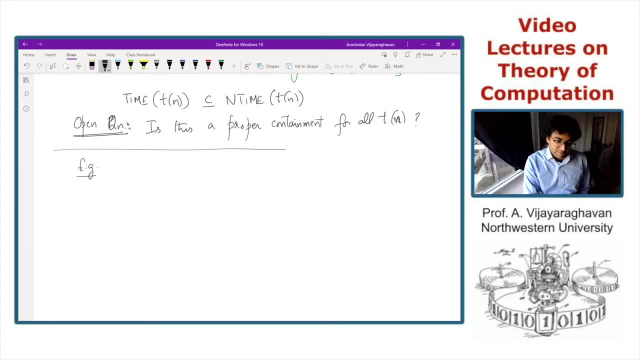 So we look at what are known as Boolean formulae. okay, over Boolean variables. This is something that you may have seen in a discrete mathematics course or a computer logic course, digital logic course. Okay now so a Boolean formulae. we'll have a bunch of variables. These are Boolean variables. Let's say: 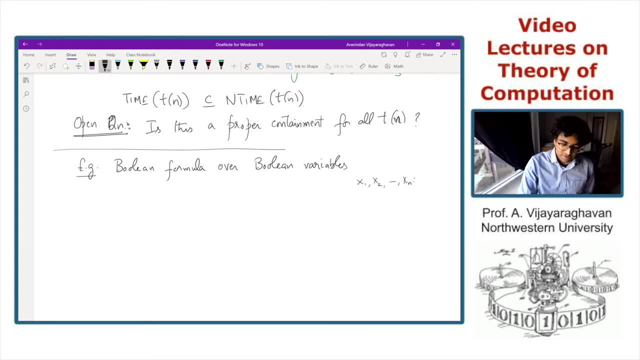 x1, x2 and so on up to xn are Boolean variables. Okay, a formulae can involve things like you know. it can involve some of these variables. you can involve negations of these variables. So this stands for, not this is and. 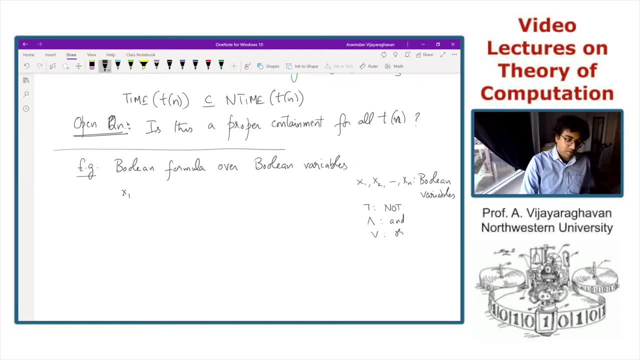 and this is or Okay. so you can have something of this form, not of x1 and x2 or x3 and yeah, not of x3, okay, and so on. Good, So you can also have brackets that tell you what's the order of operations to be done. 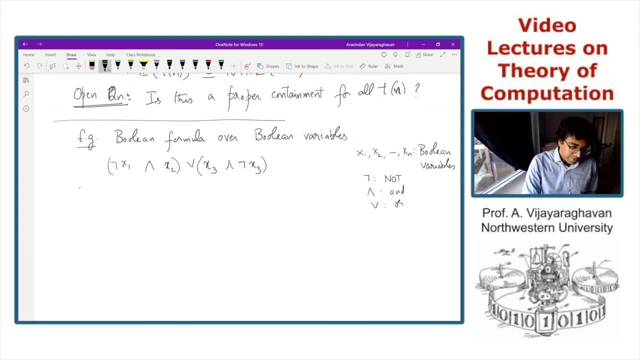 Okay, we'll say that a Boolean formula is satisfiable if, and only if, there exists an assignment, a satisfying assignment for it By mean. So by that I mean a satisfying assignment for each of the variables, so that the formula is satisfied. 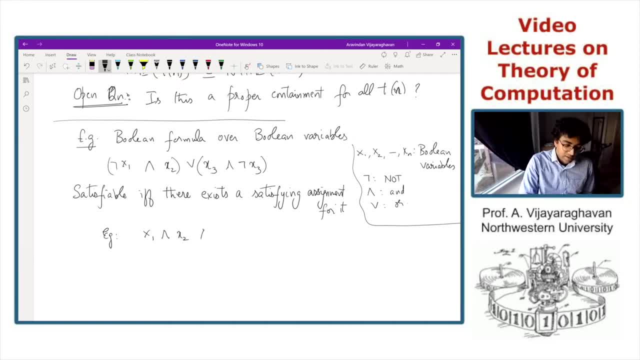 So, for instance, if you look at the formula given by x1 and x2 and not of x3,, okay, what are the rules versus if you look at another formula that's given by? maybe let me look at something a little more interesting- x1 or x2, okay, and the knot of that, followed by and of x2. 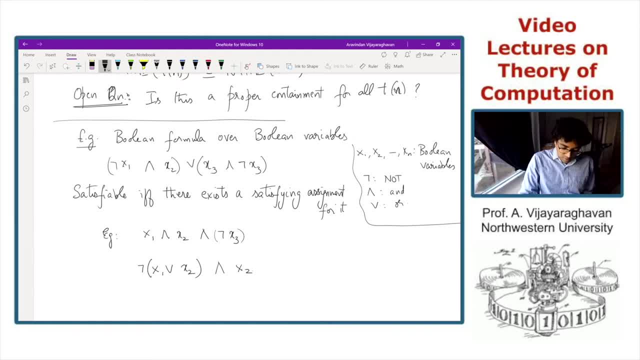 now, this is a satisfying assignment. it is a satisfiable formula. okay, because you can think of the assignment: x1 equal to 1, x2 is equal to 1 and x3 is equal to 0. on the other hand, if you think about this for a bit, this is not a satisfiable formula. 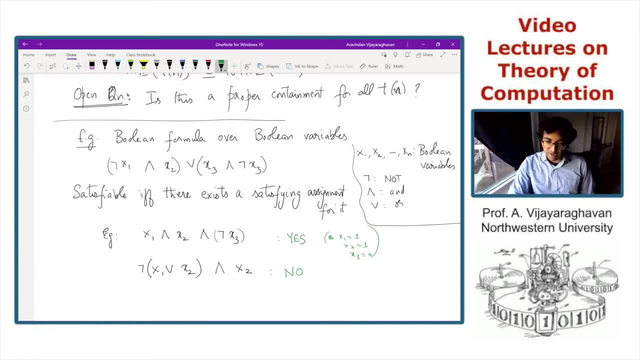 because if you take x2 equal to 1- yeah, I mean, if you take x2 equal to 1, then this second, this part, is satisfied, so it's something. and x2, so that means x2 has to be 1. but if x2 is 1, the first part is not satisfied. 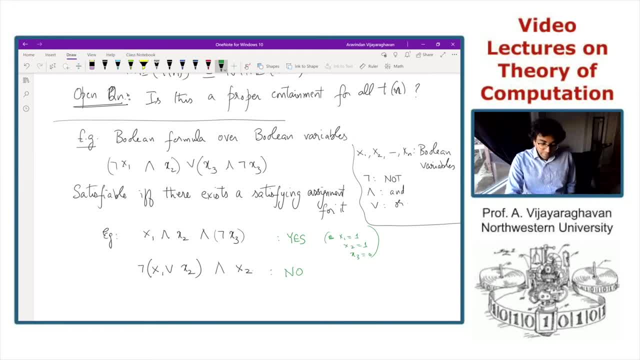 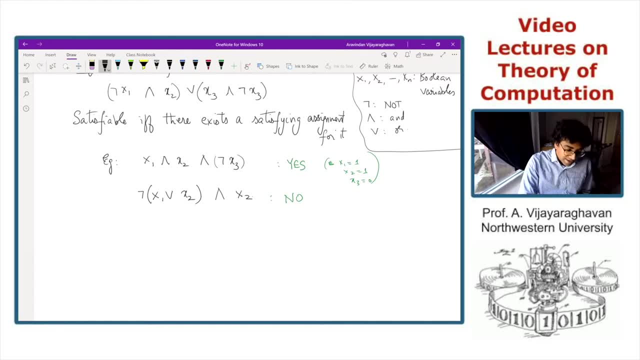 okay, good, so this is not a. this is not a satisfiable formula. good, so SAT is now a language. okay, so this is just a set of all. is a satisfiable Boolean formula? okay, the set of all satisfiable Boolean formula constitutes the class. 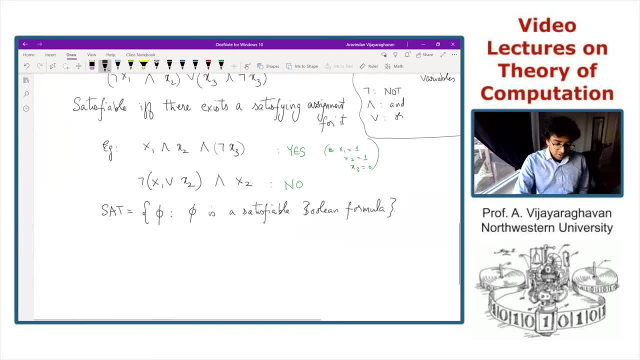 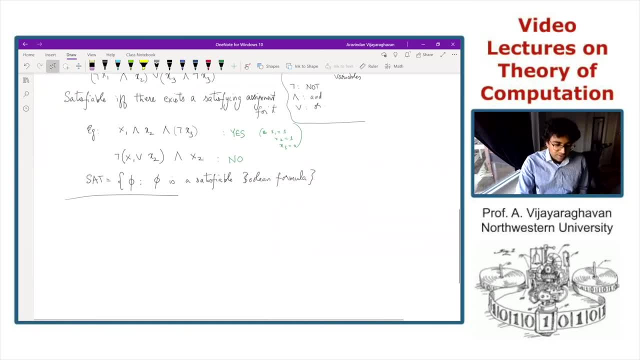 called SAT. okay, now a particular subclass of SAT that might be particularly interesting to us comes from Boolean formulae of a restricted flavor. okay, and this, this subclass of Boolean formulae, is called 3CNF. okay, the name sounds like I mean it is an abbreviation. 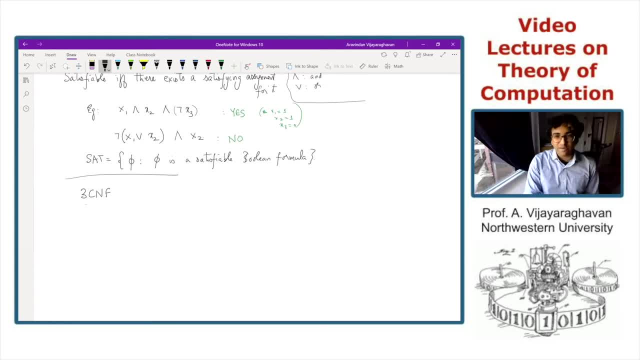 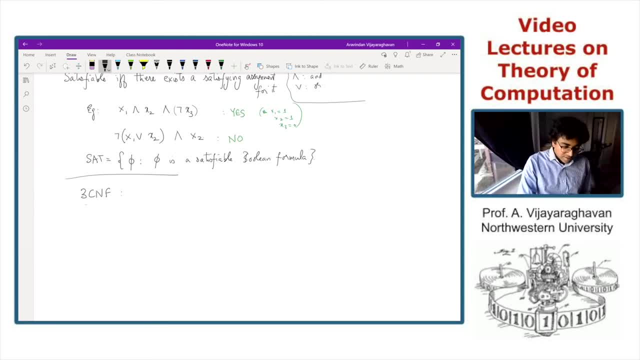 particularly in the next lecture. okay, so this consists of: it's a. I mean, it consists of Boolean formulae of a specific form. okay, so you can, for example, you may have something like this: X2 and maybe not X, X1 and not X2. 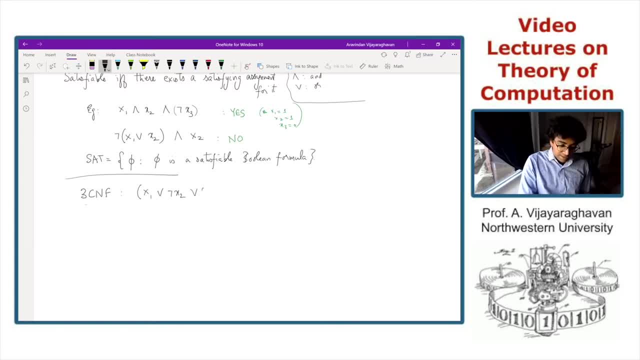 sorry or not, X2 or X3 and maybe some X3, X3 and maybe some X4 or X1 or X6 and X3 or X4 or X1 or X6 and X3 or not, X5 or not X2, and so on. 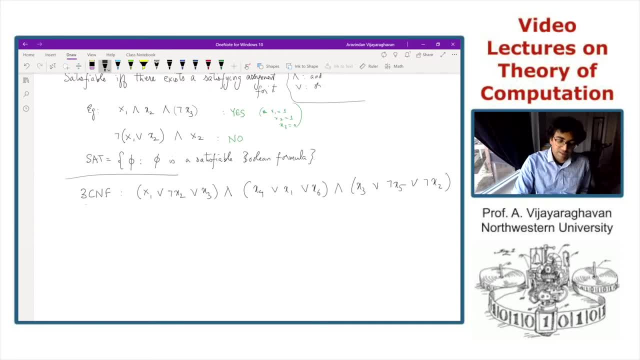 okay. so the thing to notice here is that a 3CNF formula is an AND of a bunch of expressions. okay, it's an AND of a bunch of Boolean formulae, and these individual formulae are called clauses. okay, so it's an AND of a bunch of clauses. 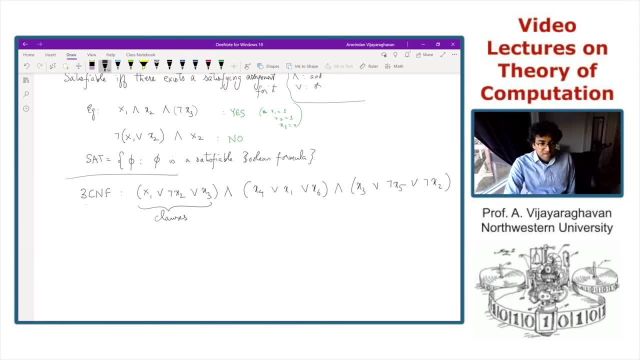 each clause is an OR of either the Boolean variables or its own negations. so these kind of things. so so these particular things. well, it's either a variable or its own negations. it's either a variable or the negation of the variable. these are called. 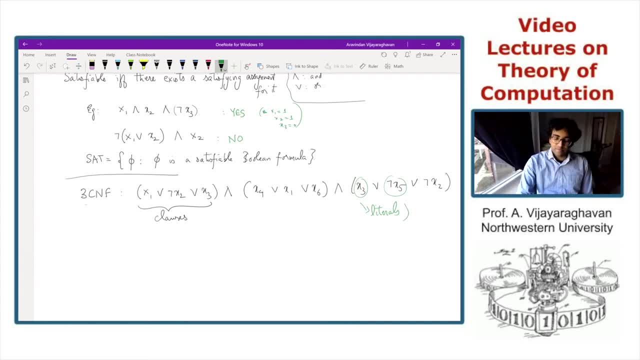 literals, okay, and these? so a 3CNF formula is just an AND of a bunch of clauses, each of which is an OR of a bunch of literals. okay, that's a Boolean. I mean, that's a 3CNF formula. and now 3SAT. 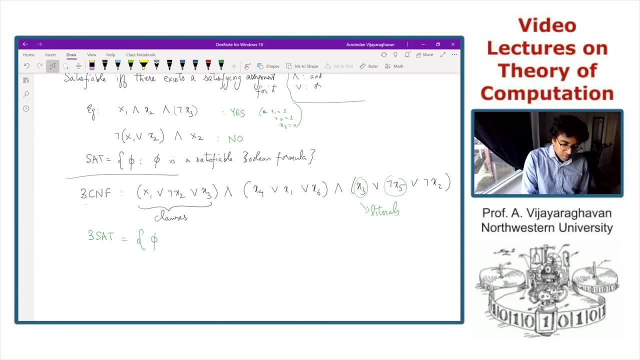 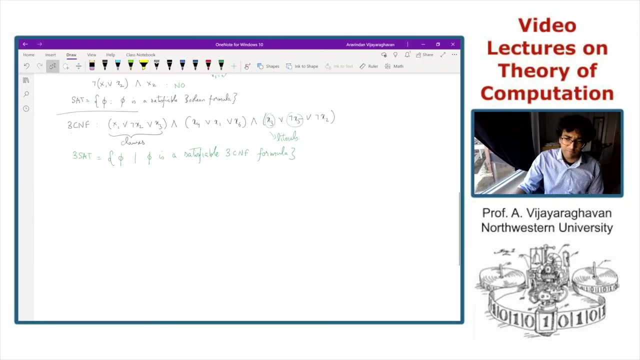 is just the set of all 3CNF formulae that are satisfiable, okay, okay. so now let's see: so 3SAT is a language and let's see a non-deterministic Turing machine. okay, an efficient non-deterministic Turing machine for 3SAT. 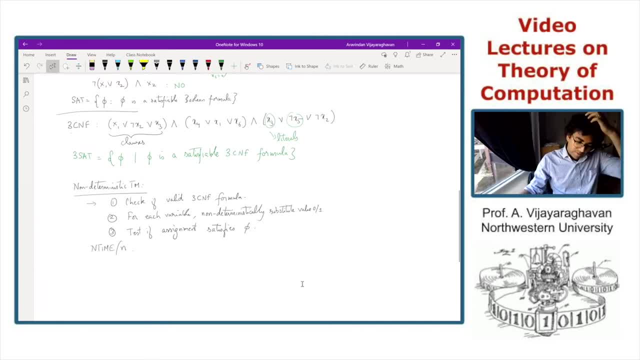 okay, let me actually just uh uh, copy paste it here. so this is a very, very simple, non-deterministic Turing machine. first given a formula phi: okay, we just on input. okay, this is on input um formula phi. okay. so, given on input a formula phi, we'll just first check. 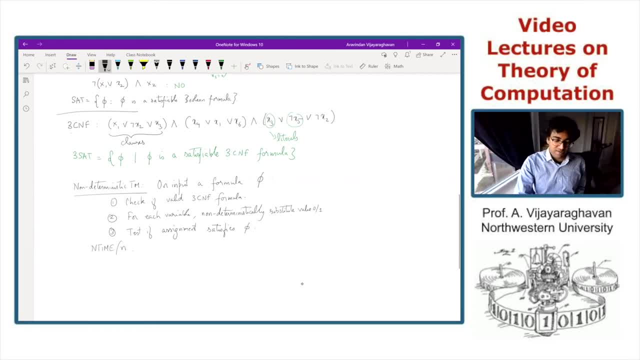 if it's a valid 3CNF formula and this just requires a scan, okay, uh, uh, you know a linear scan. okay, over the whole input. so let's say that this is a formula of, uh, an input of formula of size n. okay, that means the whole description. 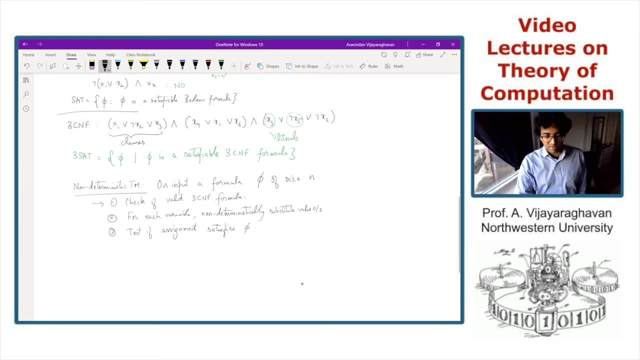 of this Boolean formula. um, you know, the Boolean formula can be described um using an n-bit strip. okay, so this includes all the clauses, the- uh, yeah, I mean how the clauses are composed of, the different variables or literals and so on, so you can check if it's a valid. 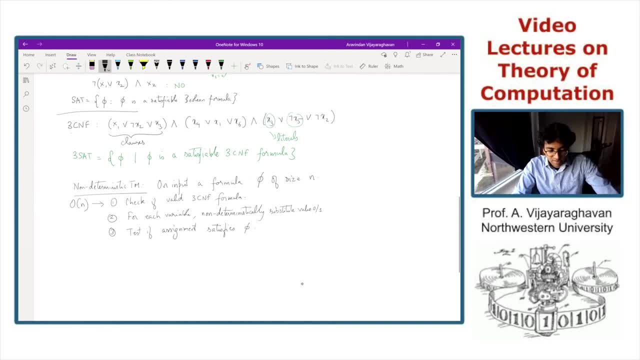 3CNF formula in just order and time, uh an, and of a bunch of odds, okay, and each of these consists of exactly each of these clauses consists of exactly three literals. so you can just go three at a time and check that it's valid and then 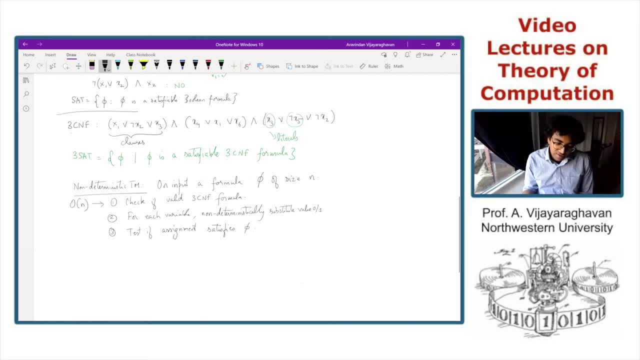 um, you know how are you gonna see if it is uh, um, um, satisfiable or not? well, for each of the Boolean variables, we are going to non-deterministically substitute either the value 0 or 1. okay, and now we'll just. this will give you. 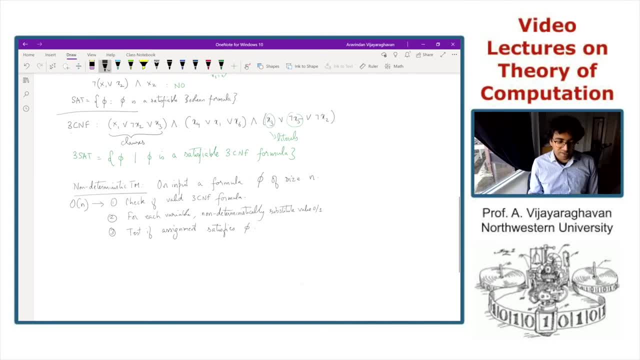 if you non-deterministically guess a value for each of the variables, then this will give you an assignment and you just check if the assignment satisfies phi. okay. so both of these steps- this is a non-deterministic step, which is order and time- this is also. 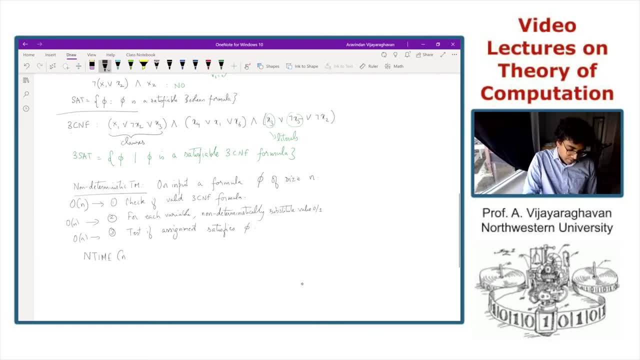 order and time. so in total this is an end time of n. so 3SAT is an end time. okay, because testing if the assignment satisfies phi is just uh, um, you know, you just need to check if all the clauses are satisfied. okay, that's again just a scan. 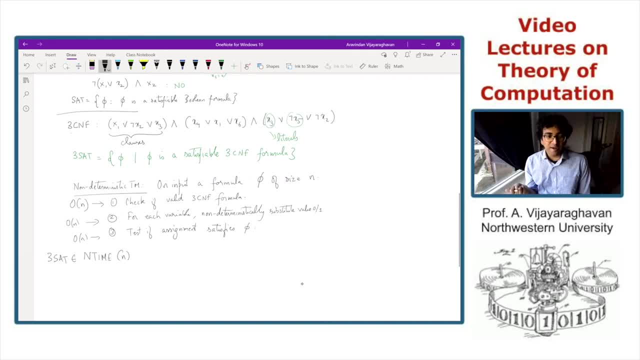 so if the formula is satisfiable, there is a valid assignment, and that is something that you would have guessed non-deterministically. now, if for all guesses it is, it is not. I mean none of the guesses. it is not a satisfiable formula, and so um. 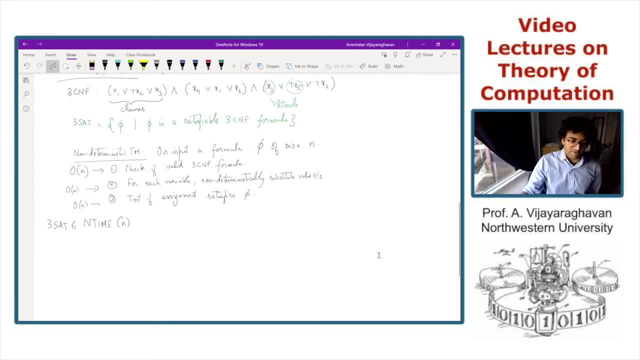 you know you will correctly reject that formula. okay, so this is an end time of n and there are many other natural problems, in fact, most natural problems that you can think about, as we will see in a bit. uh will actually fall into this class in p. okay, 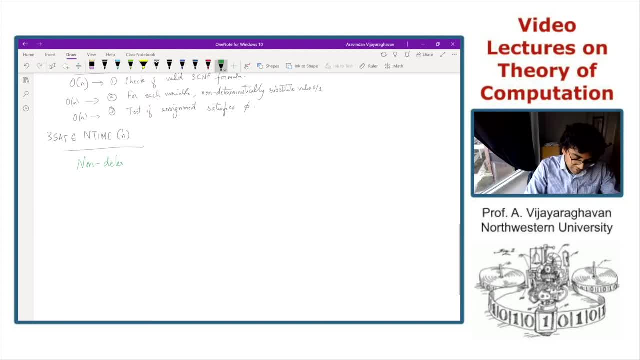 so so this is the notion of non-deterministic polynomial time. okay, so we'll define np to be just the union over all, okay, of n time of n to v, okay. so this is just, I mean basically, this is just the, I mean the non-deterministic. 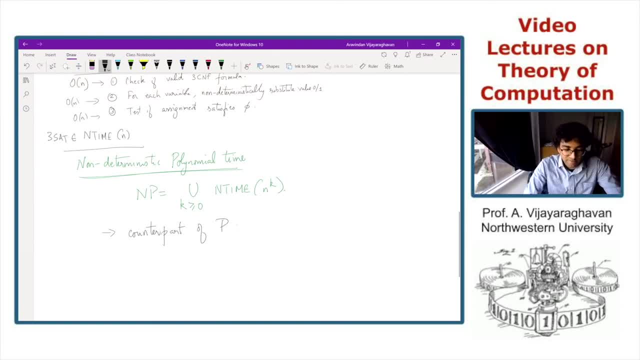 counterpart of p, which is just, you know, doing the same thing for deterministic Turing machines. okay, and this is why, uh, the complexity class time of n to the k is also sometimes called d time of n to the k, because that's deterministic and you want to distinguish against. 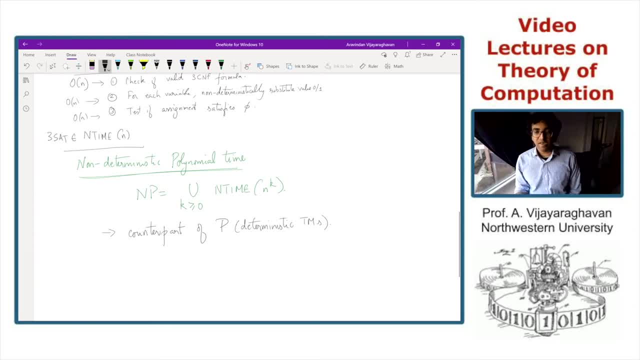 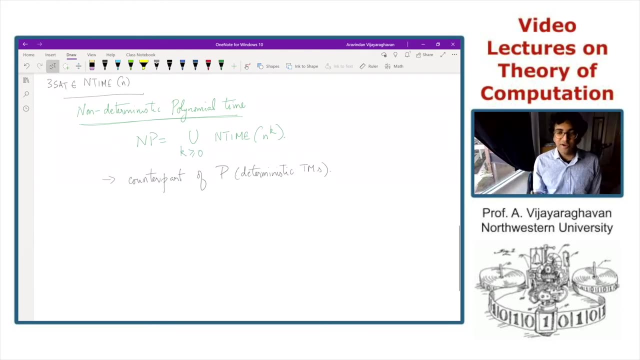 a non-deterministic counterpart. okay, so np is the set of all languages. okay, that can be decided using a non-deterministic Turing machine that takes only polynomial time. okay, so np really stands for non-deterministic polynomial time. okay, and uh, I mean, there's this misconception. 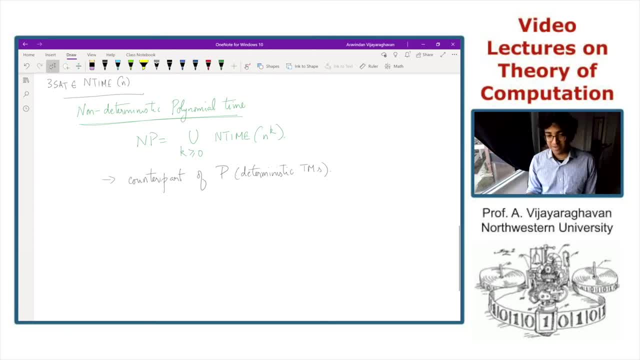 that np, uh stands for not polynomial time, and that's certainly not the case. uh, np just stands for non-deterministic polynomial time. okay, good so, but here is a slightly different, um uh, way of defining the class np. okay, so, this is a. this is a. 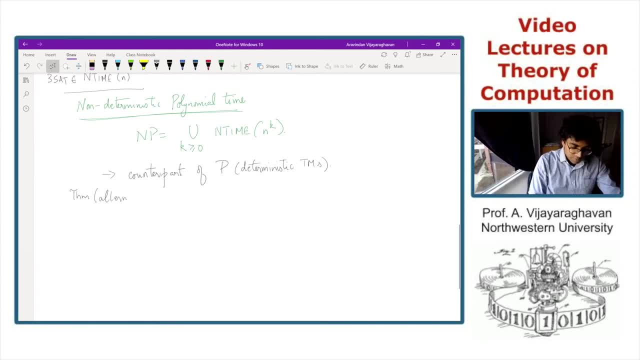 theorem, which actually also gives you an alternate definition of np, and this is actually, I mean, in many ways, this is a a more natural, or a more natural way of reasoning about the class np and uh, it's very, very useful, okay, so think about it in this way. 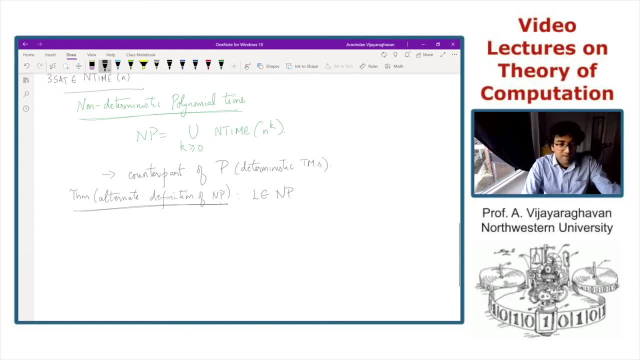 so we'll say that a language, l, is an np. okay, if, and only if. so I mean, this is sorry, this is not a definition, this is a theorem. l is an np if, and only if, there is a polynomial time turing machine, which is which we will. 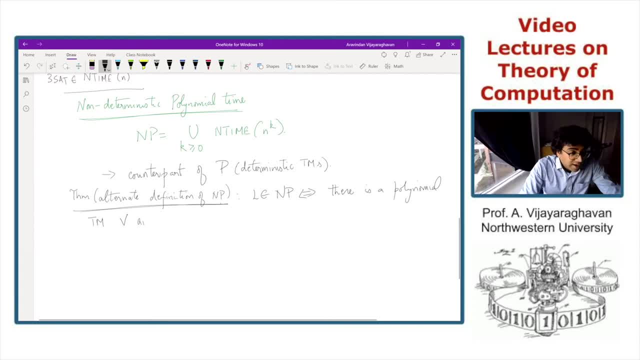 call v, okay, which stands for verifier. okay, so we can say that l is the length of x raised to the power of k. so k is this integer that's defined beforehand, and the length of y is at most, and V of X comma Y accepts. So let's just go over the statement a little bit, okay. 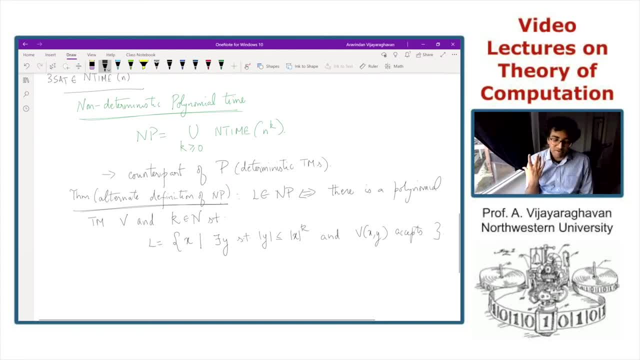 So we're saying that a language is an NP if, and only if, you can actually design this efficient polynomial time deterministic Turing machine V. So this is a deterministic Turing machine, Okay, and the number K, an integer K, is such that you know L is precisely those strings. 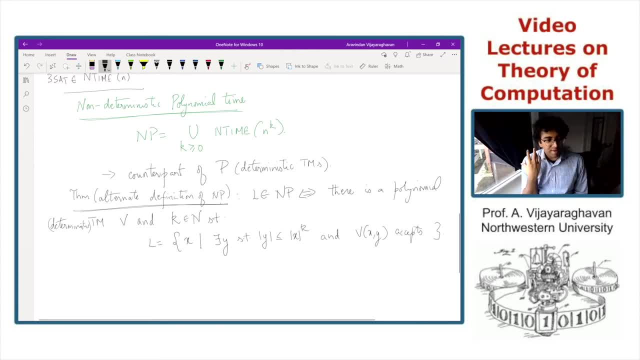 where, for every X- sorry, yeah, I mean for every X and L- you can come up with a string Y whose length is at most the length of X raised to the power of K. okay, Such that this polynomial time Turing machine V will accept X comma Y as input. 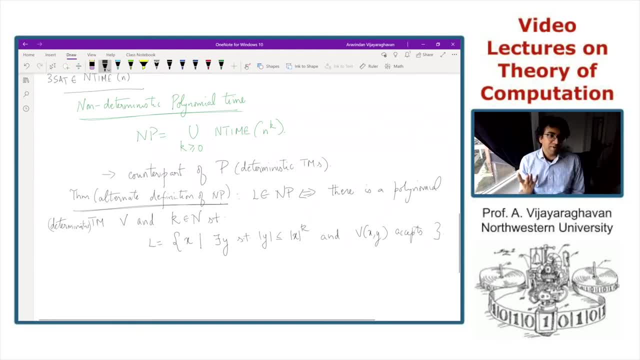 Okay, and L I mean, if you can construct this polynomial time Turing machine, V, such that L is precisely those strings X, for which there exists the string Y, which is polynomially bounded, and V of X comma Y accepts, then L is independent and vice versa. 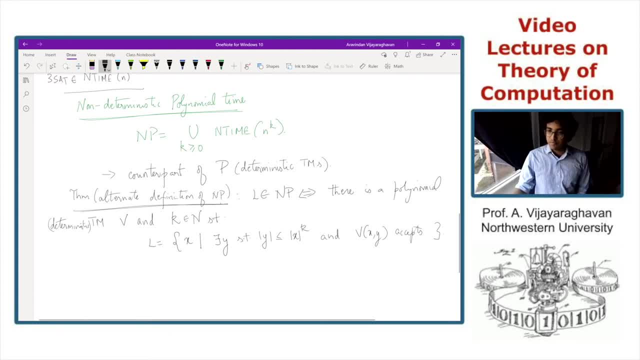 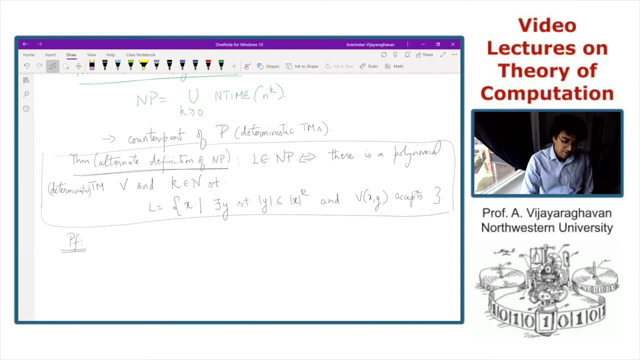 Okay, Good, Now let's prove this Fairly simple proof. okay, So let's do the first part, That is, if L is equal to the set of all strings X, such that there is another string, Y, which is of not very large size. 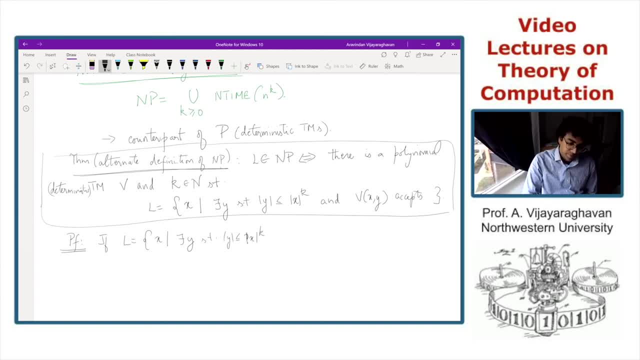 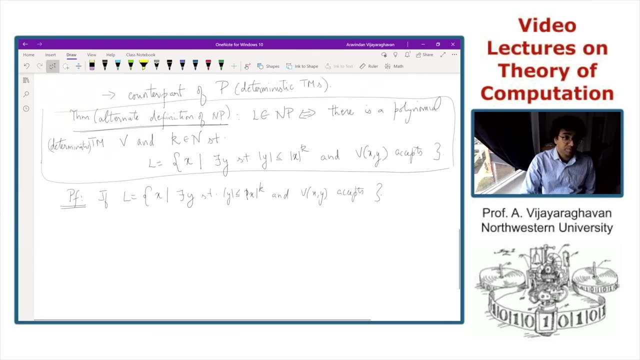 it's not a very long length, Okay. and V of X comma, Y accepts Okay. So we want to say that you know L is an NP, Okay. so how do we do this? Well, remember that V is a deterministic Turing machine. 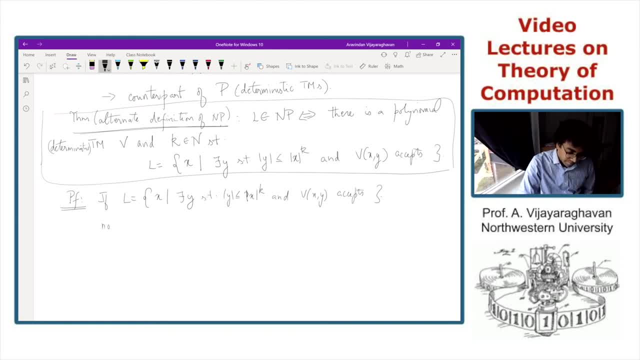 Now what we're going to do is we're just going to non-deterministically guess: Okay. so this is the first part. Okay, so we're going to non-deterministically guess Y. Okay, and we're just going to run V on X, comma Y. 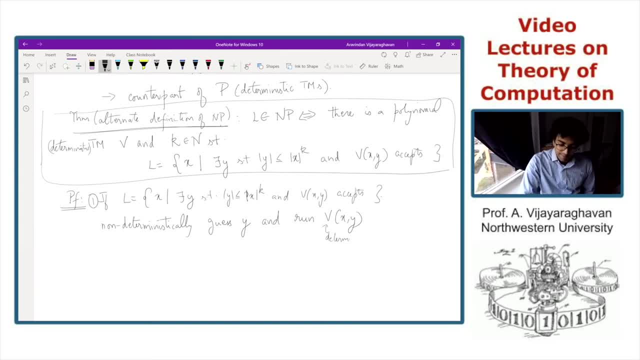 Okay, remember that this is a deterministic Turing. Okay, so, and that's it. Okay, so, this actually is the construction of the non-deterministic Turing machine. Okay, So, this is the non-deterministic Turing machine. Okay, it's just going to non-deterministically guess Y. 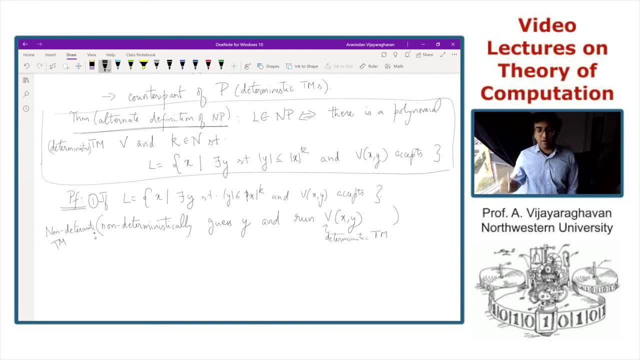 and it's going to run V of X comma, I mean V on X comma, Y, Okay, and if it accepts, it accepts X, otherwise it does not accept X. Okay, so if for no value of Y, for no guess, it is V of X comma, Y accepts. 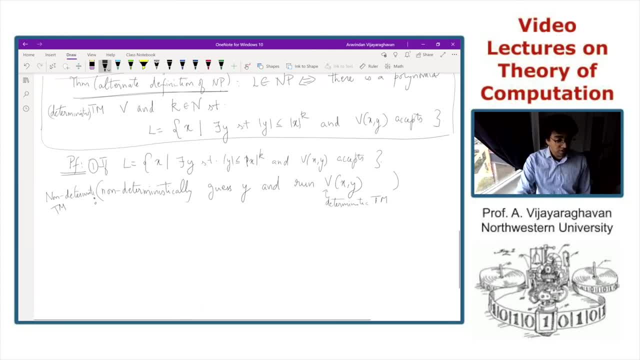 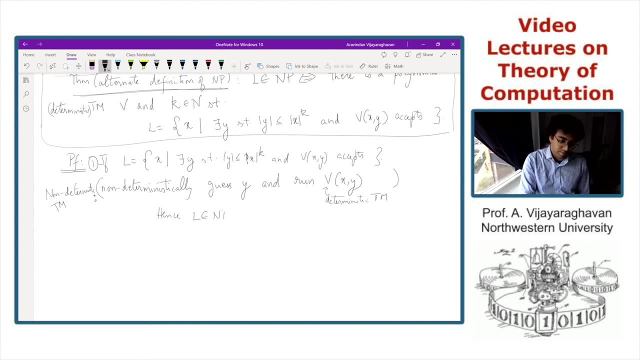 then it's going to reject. Okay, so this is a valid non-deterministic Turing machine. hence L is an NP. Okay, and the key thing to see that it is an NP is that V runs in polynomial time time for all guesses of Y. 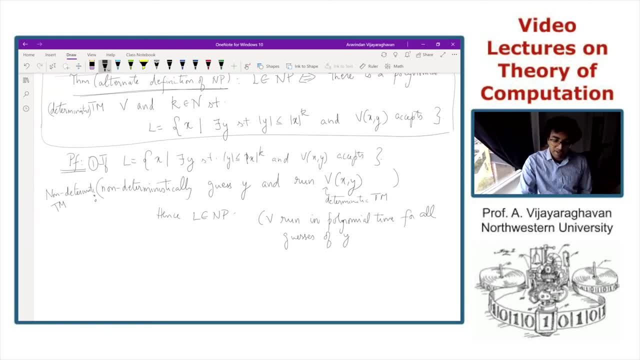 And remember that since, for all guesses, Y, since you know the size of Y, remember, is at most the size of X to the K. So this is at most N to the K and V is going to be polynomial in the N to the K. 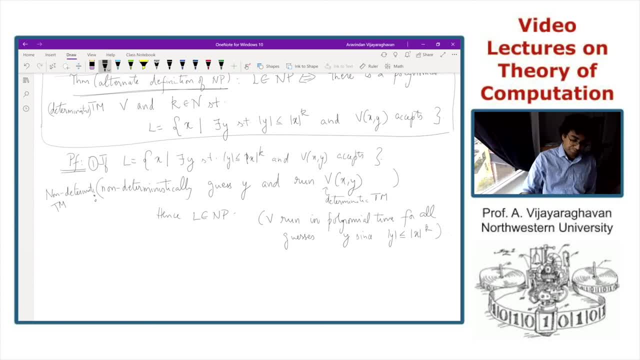 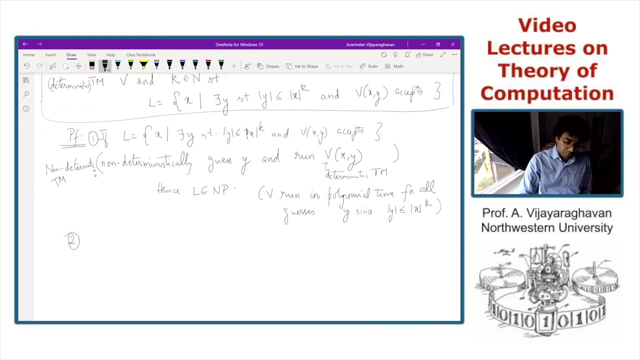 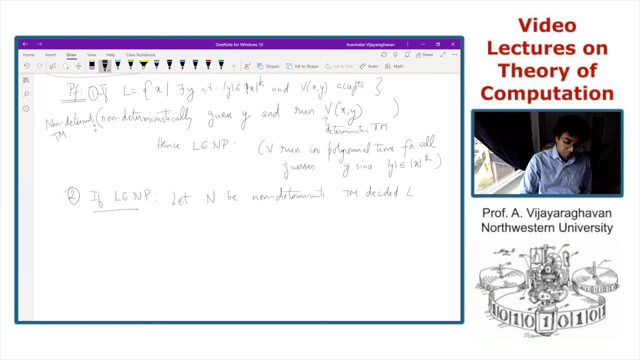 which is also polynomial. So it will be some be some non-deterministic Turing machine deciding L. Okay, now we'll define. we'll define this deterministic Turing machine during machine v, v of x comma y to accept if, and only if, y is an accepting 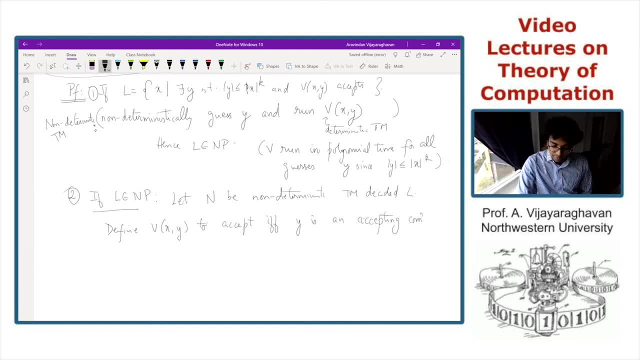 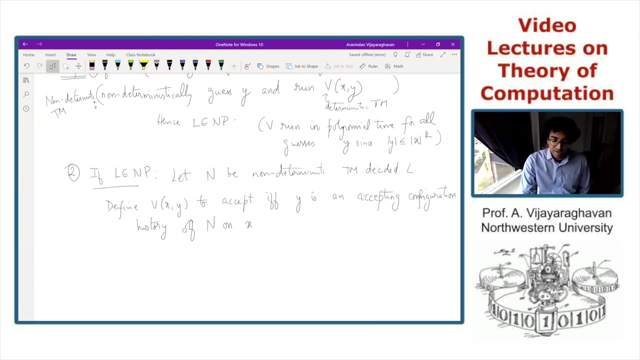 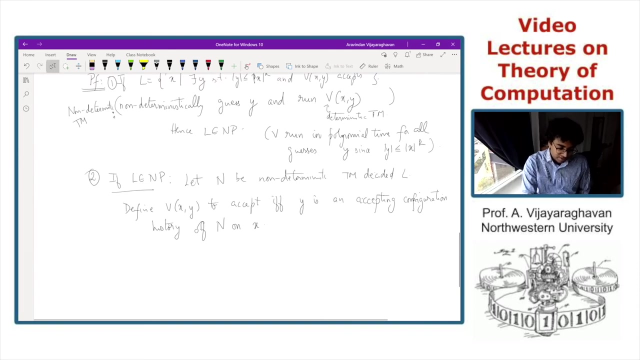 okay, configuration history or computation history for n on input x: okay, now the main thing to remember note is that checking if uh, you know, y is uh is an accepting configuration history, uh is, is quite simple to do. it's actually gonna be just uh. you know, if you remember what accepting configuration history is, it's just a sequence. 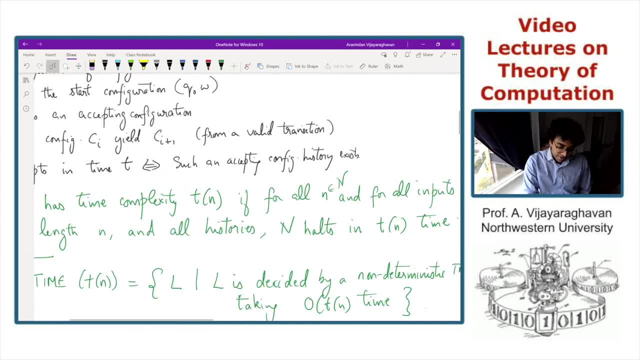 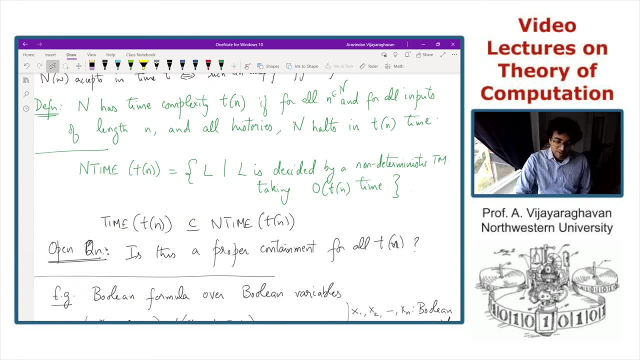 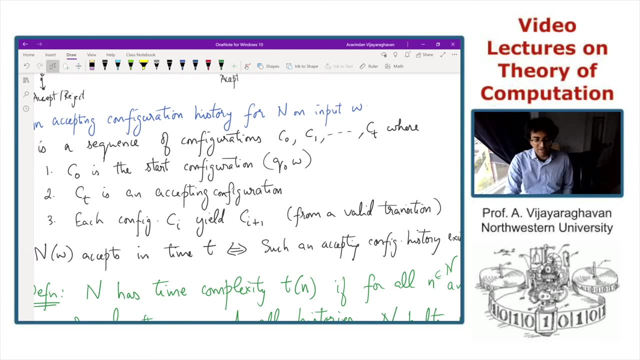 of configurations. okay, where, uh, the starting configuration is going to be, uh, you know the start state, comma w, and then you know each ci in ci plus one through a valid transition or valid move, and then you finally have to reach an accepting configuration. so you just need to go and check if each of these 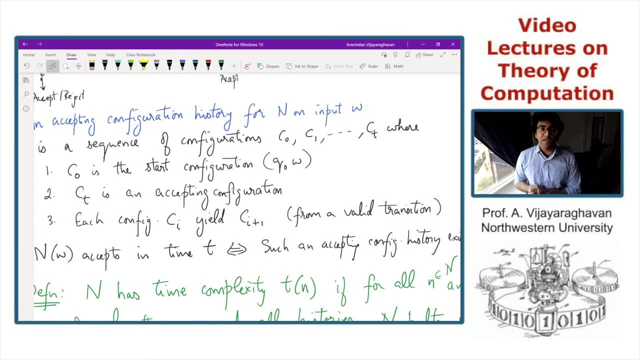 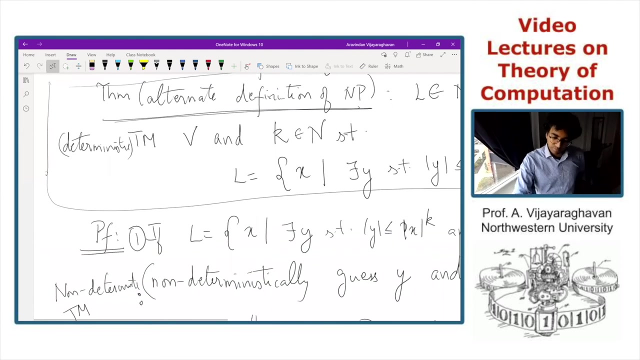 successor configurations correspond to a valid transition. okay, and this just requires going through each of these configurations and checking that they're valid, and you start from a c0 and you end up in a valid accepting configuration. okay, so this can be done efficiently. and so now, um, okay, so this is hence. 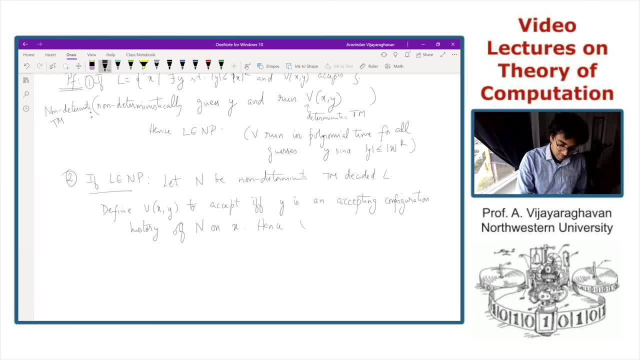 um. so this, this actually concludes state curing machine that we need, and this shows that uh, uh, you know you can actually write it in the same form. okay, so l is also. this says that l is, uh, the set of all x's, such that you can come up with the y? um, which is not too big. okay, that? 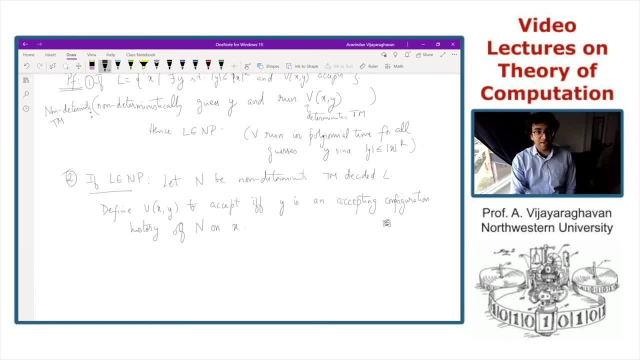 corresponds to the configuration history, such that v of x comma, y, xx okay, and y is y small. this is okay. just to uh, elaborate a bit more on it, y is y small, y corresponds to the length of y. okay, corresponds to okay. um, and we know that this is polynomial because it's an np. 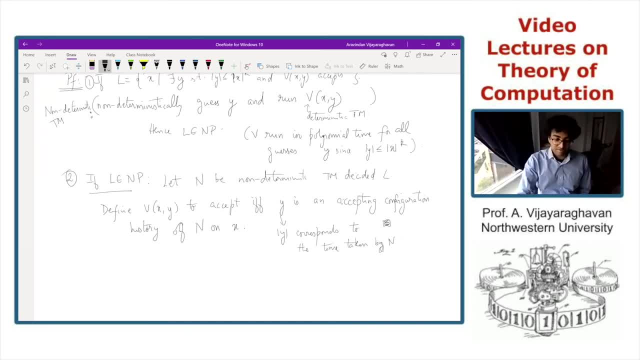 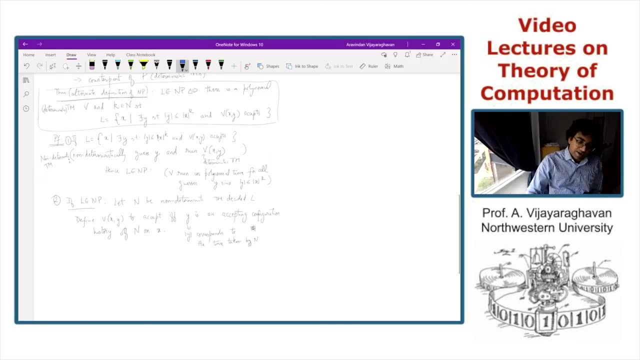 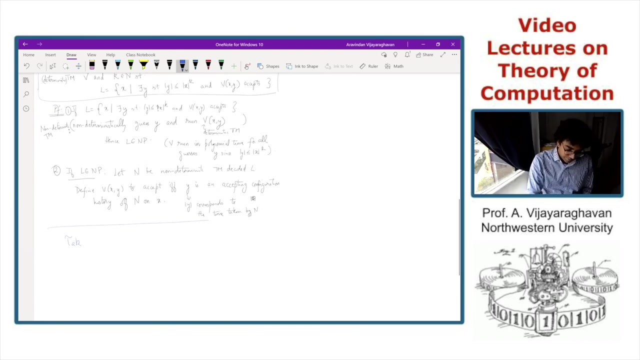 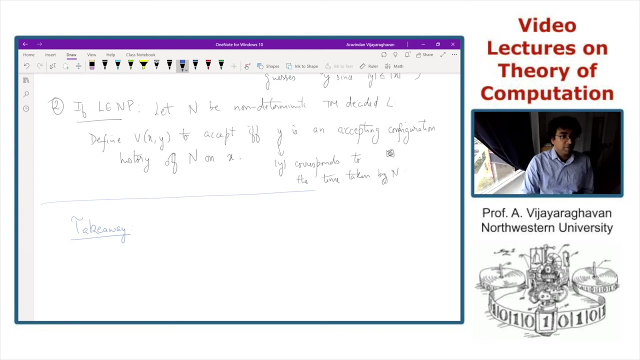 okay, so y is also small and uh. so this, uh, this gives you what you want. good, so you have this alternate definition of the class end. i would say that the main takeaway is this: alternate uh characterization or view of np. okay, and so you can say that a language, l, is an np. 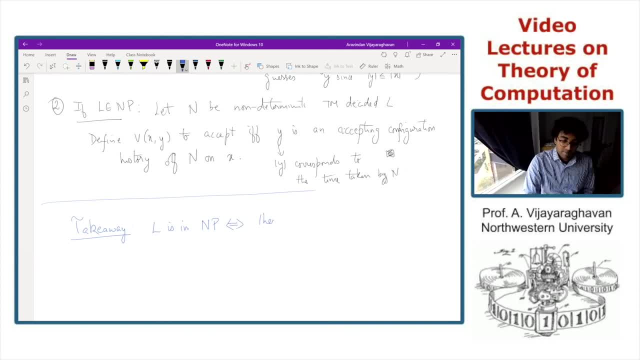 if, and only if, there are polynomial length proofs. are certificates of membership? okay for l verses. okay, i will just wait for a second. okay, are there any other questions? okay, let me use this. okay, this will give me a lot of potential homo, And not only do you need to produce this proof y. 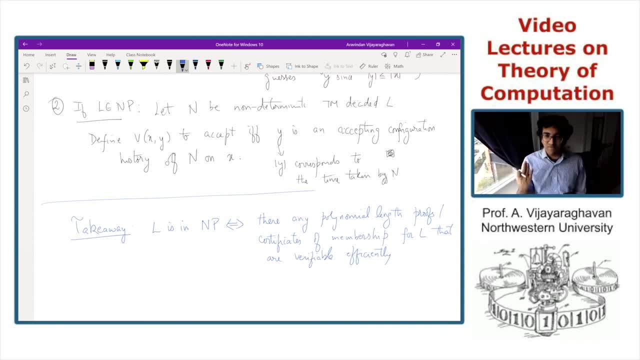 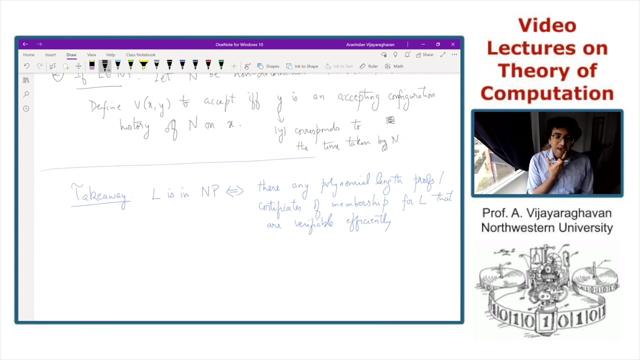 you also need to check that. there is some efficient procedure, which is the steering machine v, that can look at x and y and tell if that accepts, based on whether y is a valid proof or a valid certificate for x. So good, So those languages in NP are exactly those languages. 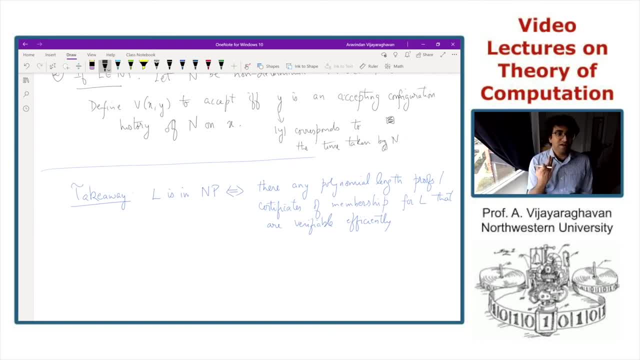 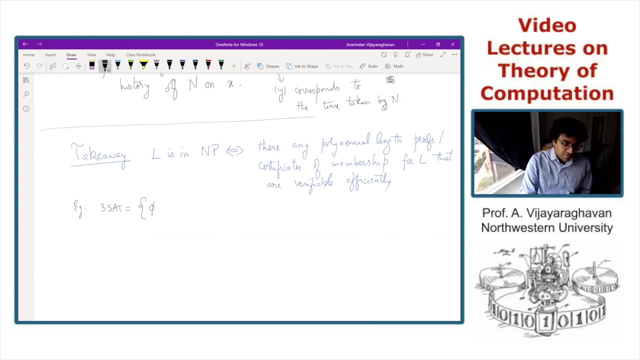 for which there is like an efficiently verifiable proof of membership, So for example, 3SAT. so let's just write down 3SAT in a way that makes it clear that that is such an efficient certificate. So it's just a set of all formulae v. 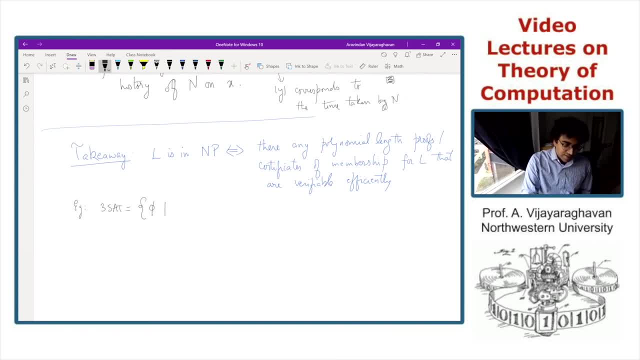 Boolean formulae I mean, which are 3CNF, such that phi is 3CNF, such that there exists a y, such that y is satisfying. So I'm just going to write down the assignment to phi, OK. 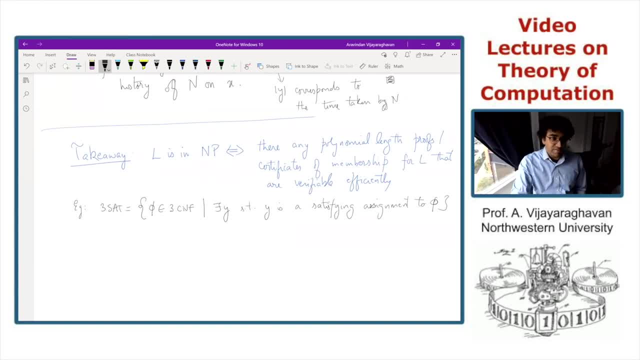 So the fact that phi is a 3CNF formula is easy to verify. OK, And in fact, if you want, I can actually write it here. OK, That can be easily verified. But yeah, so 3SAT exactly corresponds to those 3CNF. 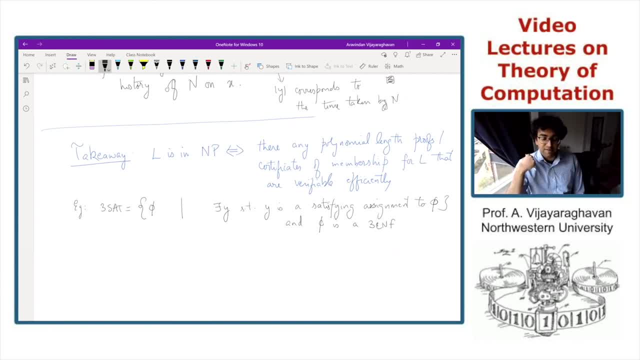 formula such that there is a y which is a valid satisfying assignment. So y is just proof that the formula is satisfiable. It's just a satisfying assignment. OK, so 3SAT is an NP. We already saw that it was an NP. 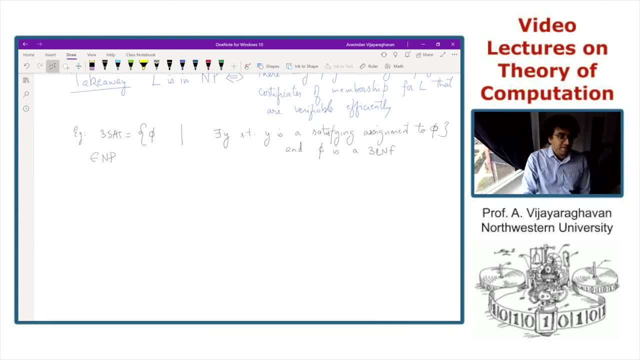 but there's an easy way to see that it's an NP And most natural problems that actually you you would encounter are actually an NP. So some examples are: clique: These are problems that you might see in a future class on the algorithms class of Hamilton path. 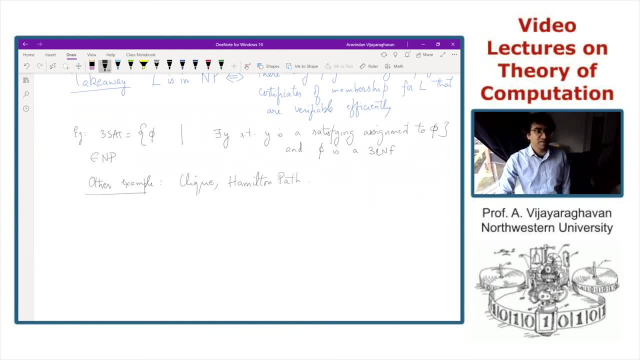 And in fact, many of the problems that we care about, actually fall into this class NP, Because these are the problems for which, even if you have a solution, I mean you should be able to mean the basic requirement for computational problem that I mean you may care about. 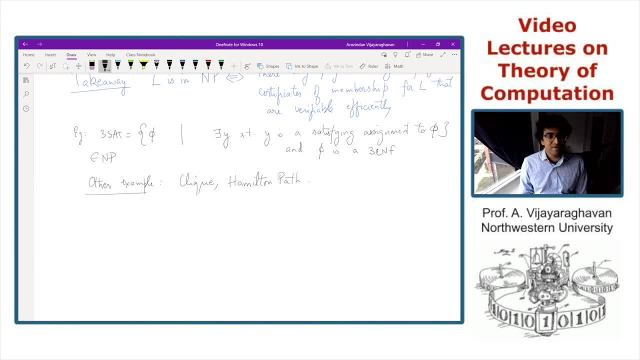 is that when you see a solution, you should be able to verify that it's a solution, And NP exactly captures all those problems. OK, good, So let's just recap what we have seen in the last two lectures. So P is the problems, the set of all problems. 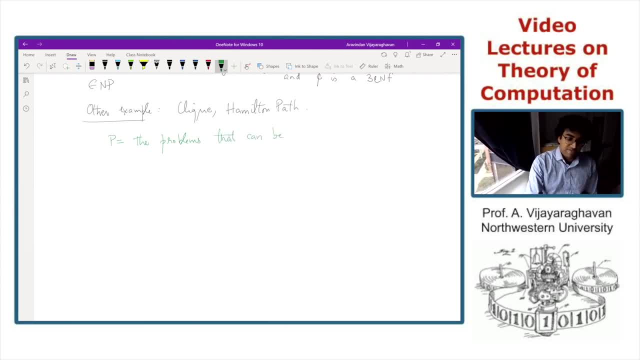 that can be efficiently solved. OK, by efficiently solved, we mean solved in polynomial time. NP is the set of all problems where proposed solutions can be verified efficiently, And NP is the set of all problems where proposed solutions can be verified efficiently- OK. 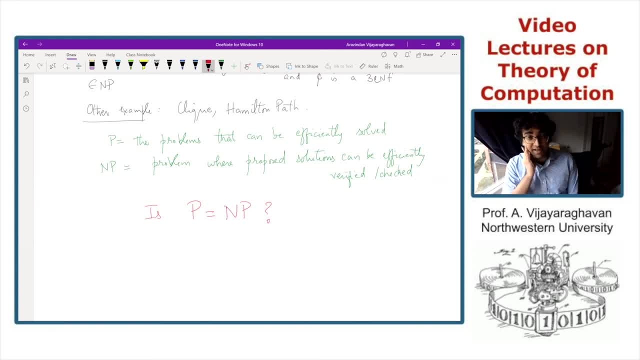 And a million-dollar question is: is the class P equal to NP? It's literally a million-dollar question because this is one millennial problems that were identified by the Clay Institute And it's a profound problem with many, many philosophical implications. 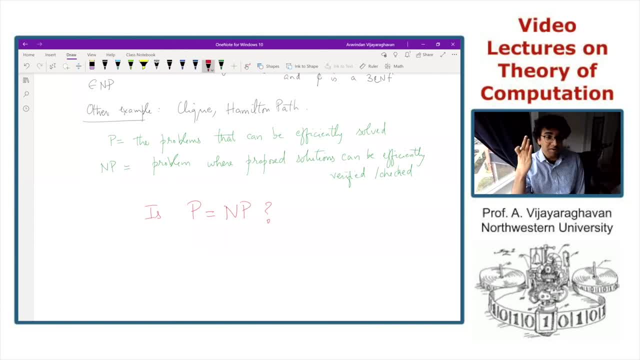 But let's just again see what it is. So P is the set of all problems for which we do have polynomial time algorithms. So this is a notion of efficiency. You can solve it efficiently. NP is a set of all problems where given a solution. 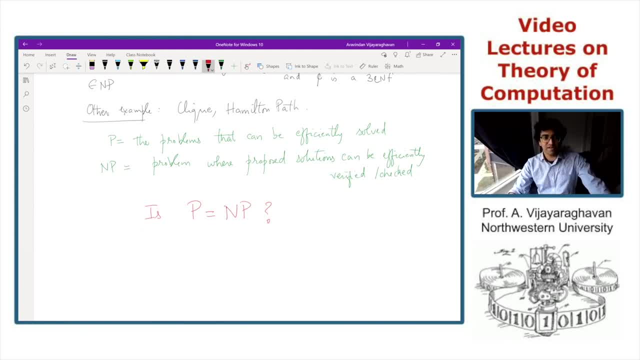 I can verify in a proposed solution. I can verify if it is efficiently, whether it is a solution or not. You can identify a solution efficiently. I mean identify a proposed. I mean verify a proposed solution efficiently. Now the P versus NP question basically asks: 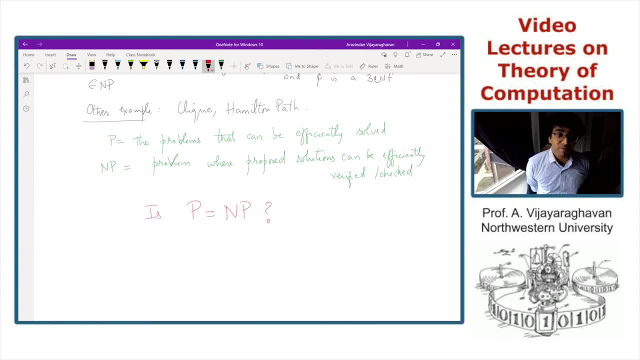 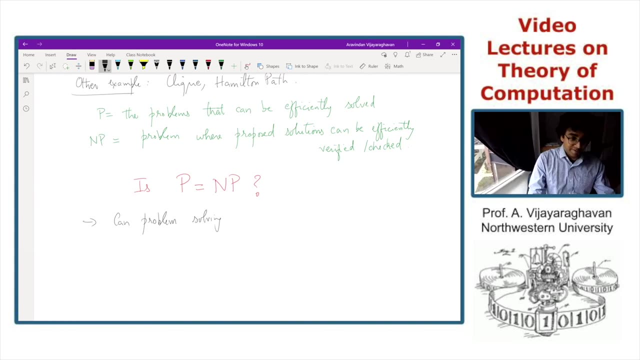 well, if you can verify a proposed solution efficiently, can you also find one, So it's. I mean so it's related. It's related to things like: can problem solving be automated? Because if you can verify a solution to a problem, 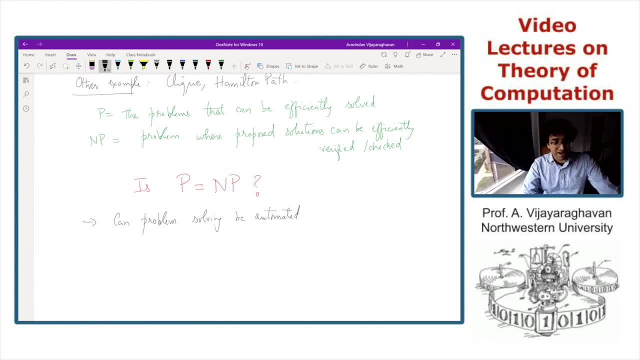 efficiently. can you in fact end up? I mean, can you actually go ahead and find one, find a solution efficiently, And it also has many other? I mean, if P is equal to NP, it will have major consequences. 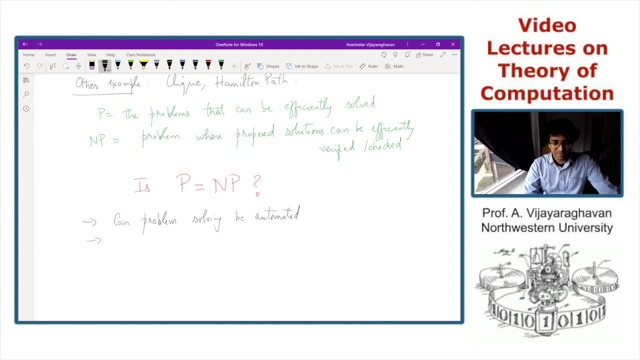 I mean I mean profound consequences, Like you can automatically prove true theorems, true statements. I mean it is also related to things like automating creativity, because I mean NP really captures all those things where that you can recognize.